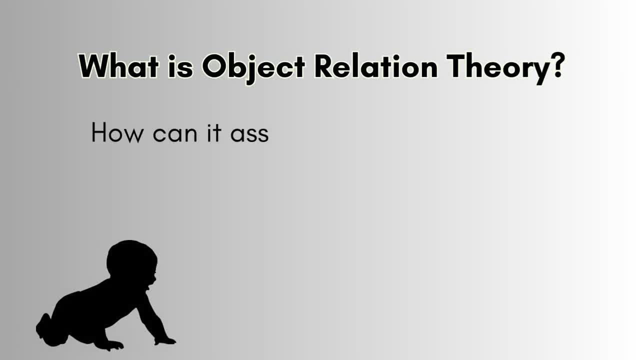 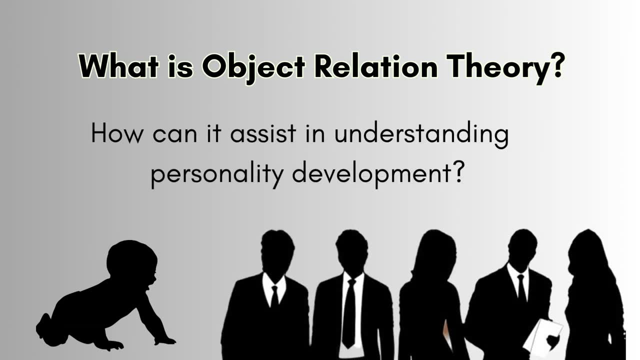 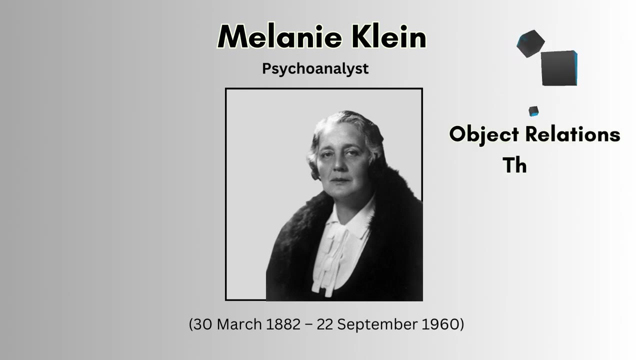 In this video, we take a brief look into the workings of Object Relations Theory and discover how it can help us to understand the developmental mechanisms behind our personality. Melanie Klein, an Austrian-born psychoanalyst, was the originator of Object Relations Theory. She developed this based on her clinical work with children and adults and her observations. 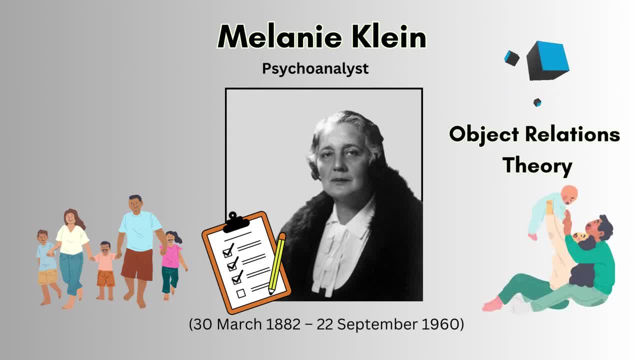 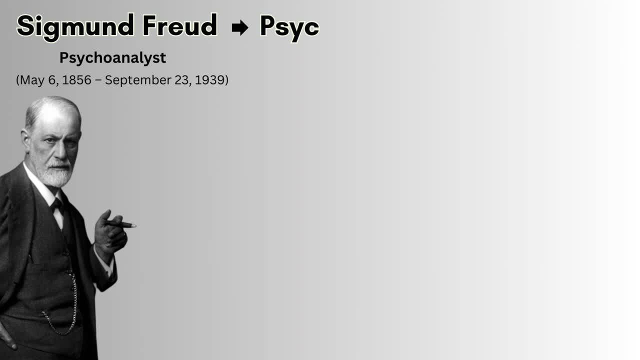 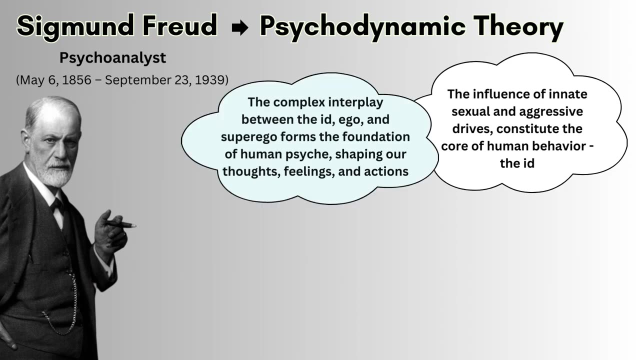 of early parent-child relationships. Her theories, which were considered controversial at the time, differed from that of Freud's and brought forth new perspectives on child development. Freud focused on innate drives and intra-psychic conflicts. Freud proposed that child development occurs in a series of psychosexual stages: oral, anal. 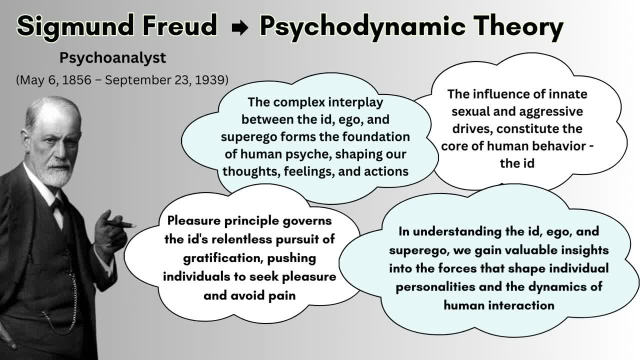 phallic and latent, as well as the genital stages. Each stage is characterised by the focus of libidinal or sexual energy on different erogenous zones of the body. On the other hand, Klein believed that the early interactions between infants and their 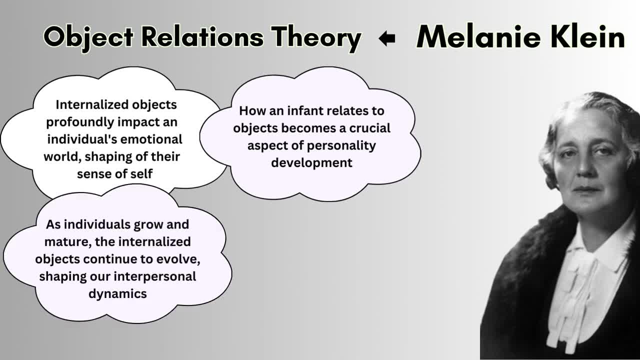 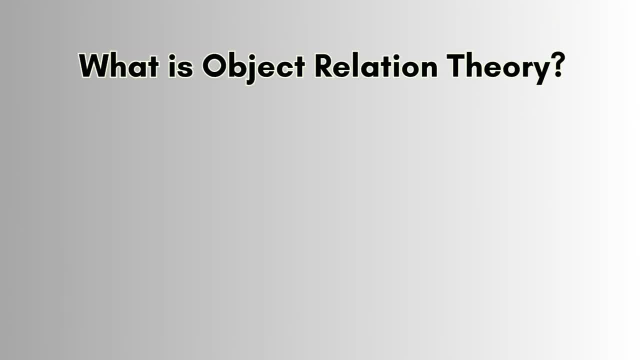 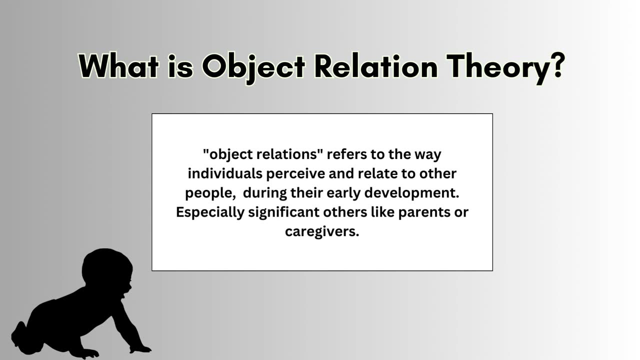 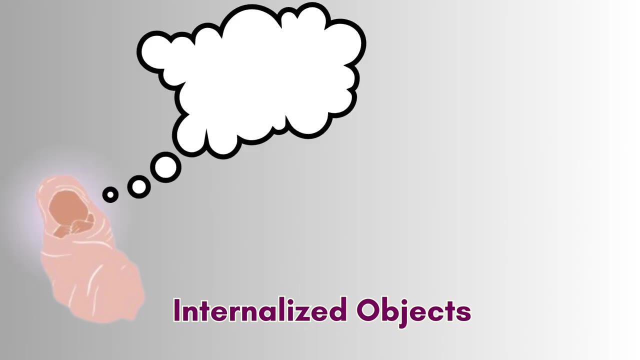 caregivers profoundly shaped their internal world and laid the foundation for future emotional development and relationships. In a nutshell, Object Relations refers to the way individuals perceive and relate to other people during their early development, especially significant others like their primary caregiver. She introduced the concept of 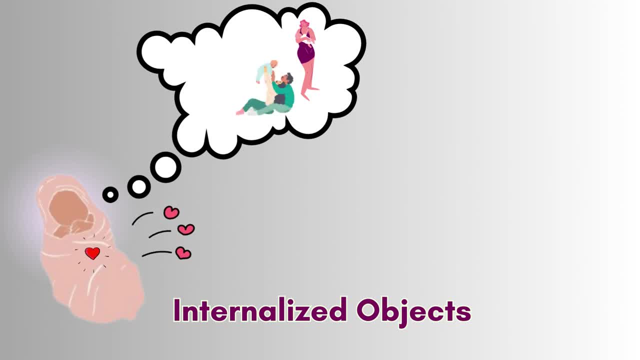 internalised objects which reside within the individual's psyche and influence their emotions and behaviours. These objects are mental representations of important people in an individual's life, in particular their primary caregiver. These representations can also include parts of a person or objects from one's inner-world, For example, an individual. 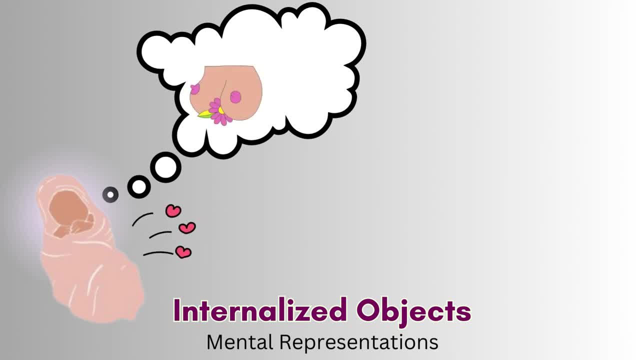 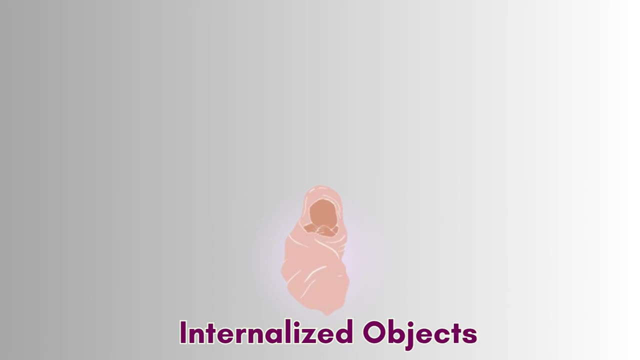 may relate to the symbolic meaning of the breast as a source of nourishment and comfort, which then becomes part of their internalised image of their mother. These internalised objects influence emotions, attitudes and behaviours in relationships throughout life. The internalised representations or mental images that the infant experiences in relation to their primary caregiver. 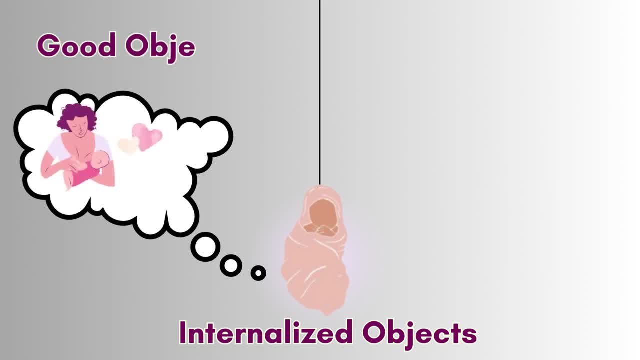 fall into two main categories: good objects and bad objects. Good objects, in object relations theory, represent the positive and nurturing aspect of an object, especially the primary caregiver. They are formed based on experiences of comfort, care and emotional support, leading to feelings of security, love and trust. 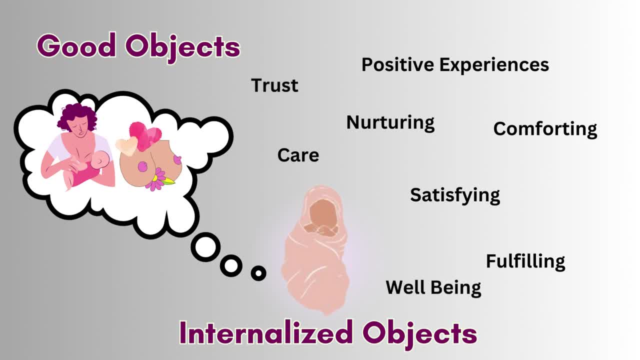 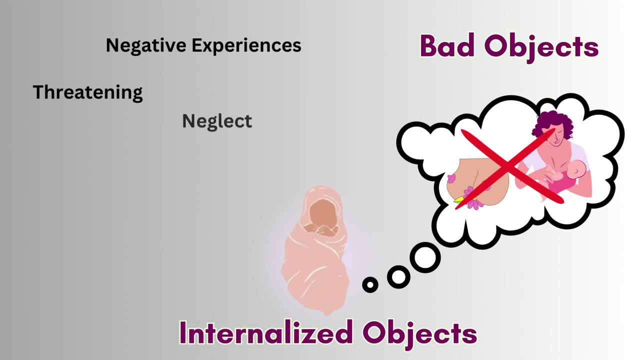 Good objects serve as sources of comfort and emotional nourishment, contributing to the individual's wellbeing and positive attachment experiences. Bad objects, on the other hand, symbolise the negative and threatening aspects of significant others or the primary caregiver. They arise from experiences of frustration, neglect or perceived harm from the caregiver. 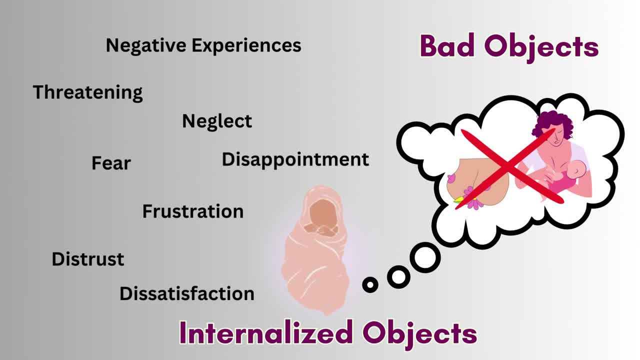 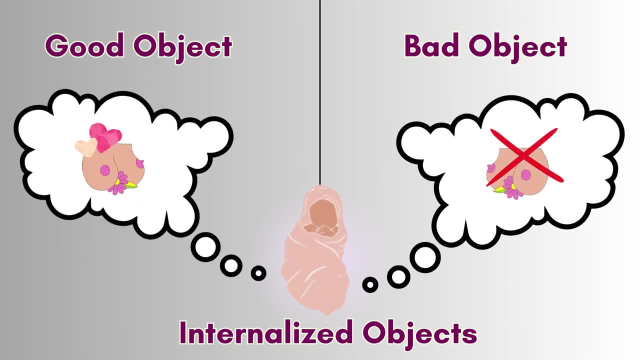 leading to feelings of anxiety, fear and disappointment. Within the infant's mind, the same object can be represented as a good object and a bad object. For example, when the mother speaks, the baby's breasts are full and the baby is getting nourished. 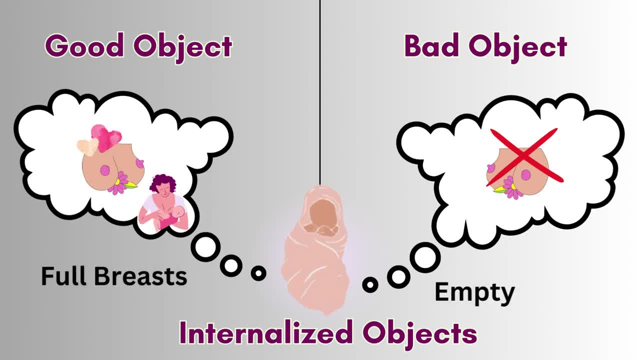 the mother may be perceived as a good object. But when the mother's breast is empty and the baby is left feeling hungry or dissatisfied, the mother may be perceived as being a bad object. In object relations theory, the process of a child's relation to good objects and bad objects in early infancy. 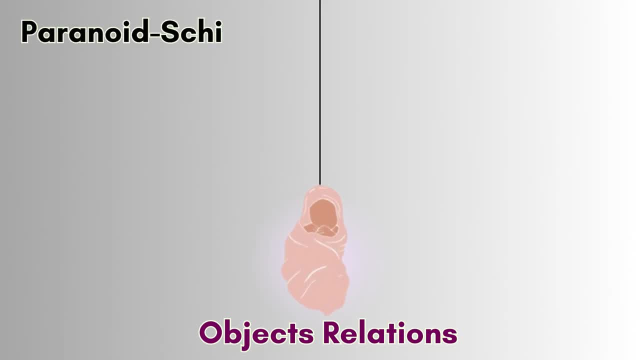 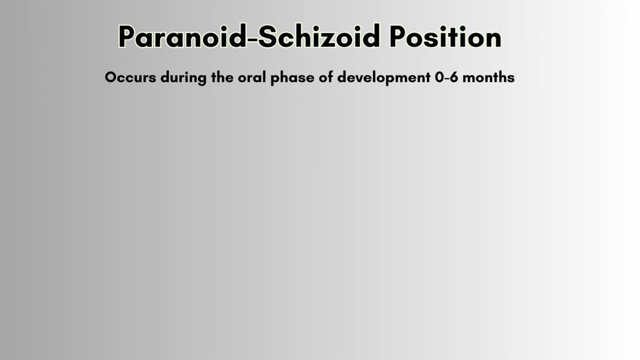 is described through two main positions: the paranoid schizoid position and the depressive position. These positions represent different stages of emotional development and how infants perceive and relate to the world and their primary caregiver. During the paranoid schizoid position, infants in this stage are primarily driven by primitive emotions and impulses. 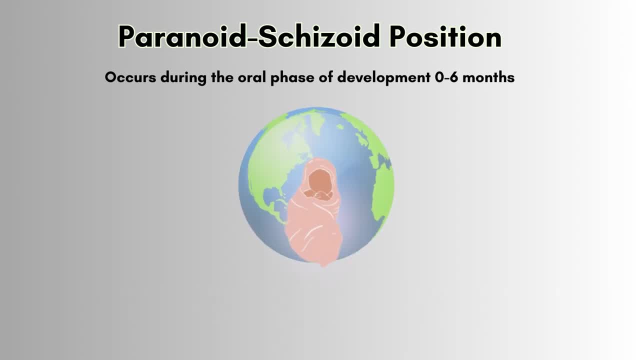 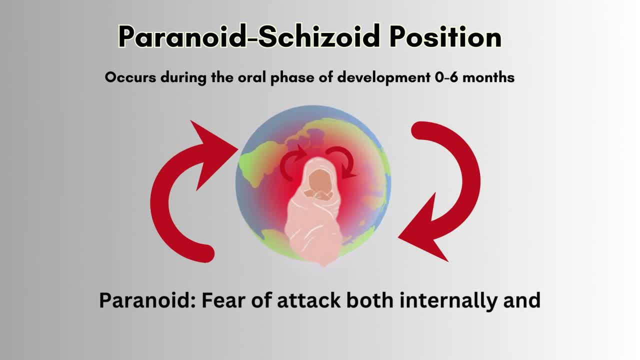 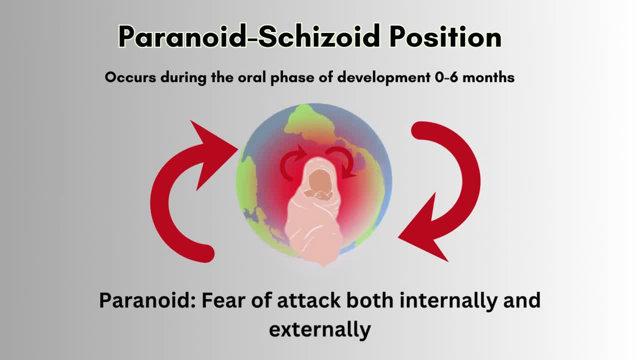 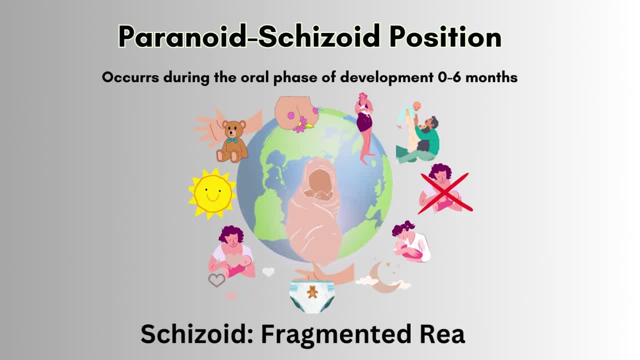 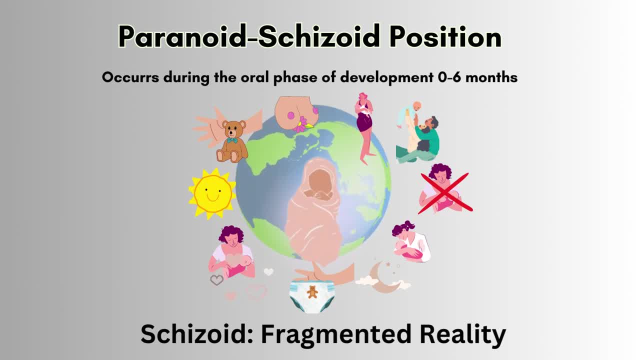 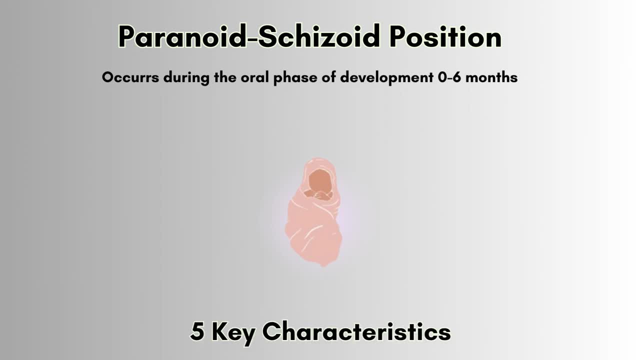 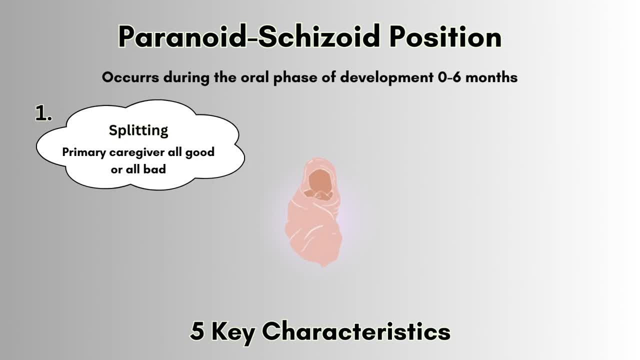 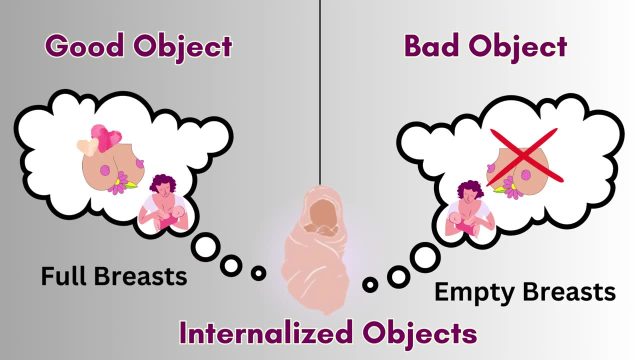 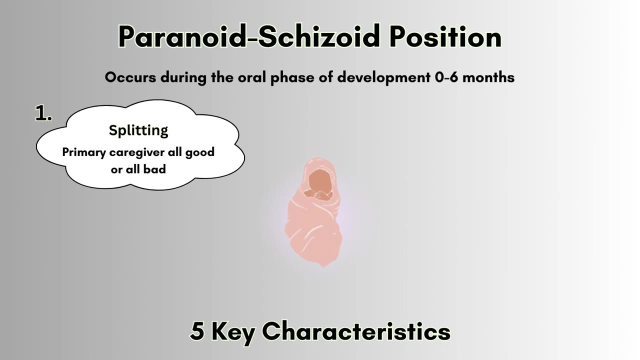 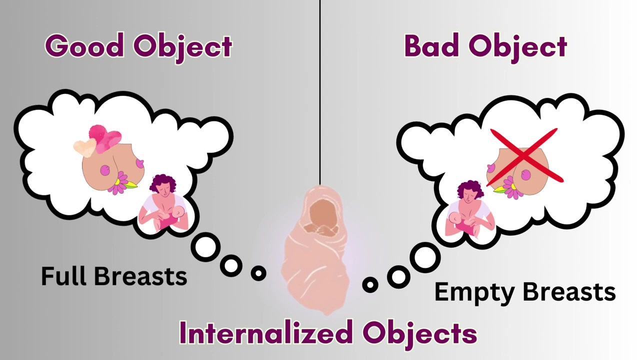 where the infant experiences the world in a fragmented and polarized manner. they tend to split the experiences into good and bad, without integrating both aspects. this splitting also applies to their perception of their primary caregiver, whom they may see is either entirely loving and nurturing, like with the good breast or the good mother, or it's highly harmful and withholding, like 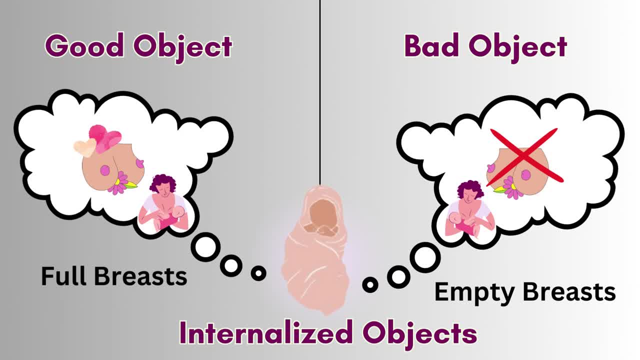 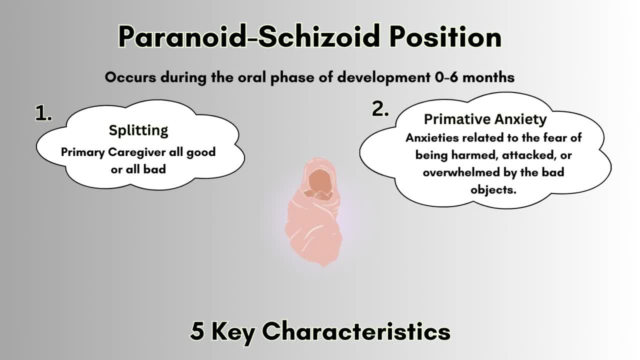 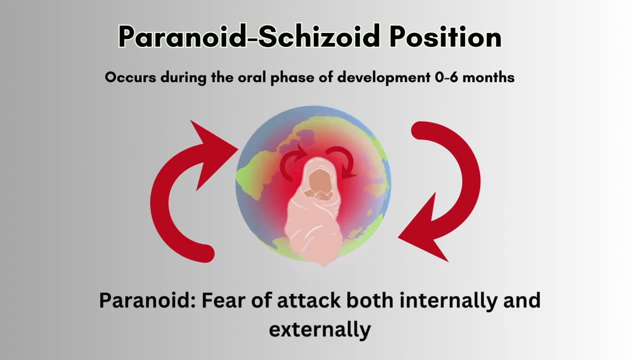 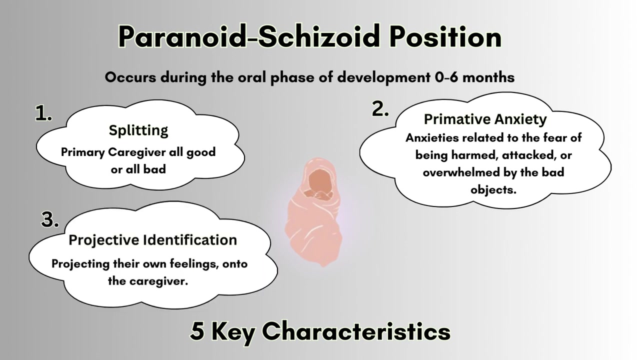 the bad breast or the bad mother. another characteristic feature is primitive anxiety. in this position, the infant may experience anxieties and paranoia related to the fear of being harmed, attacked or overwhelmed, or by the bad objects or caregivers. they may also experience fear of annihilation leads into a basic need for survival and protection. the infant may engage in. 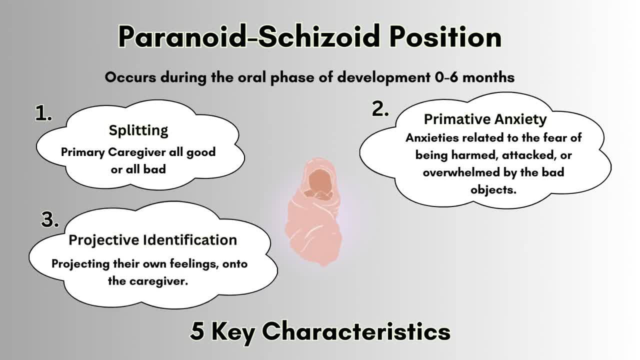 projective identification, a defense mechanism where they protect their own feelings, particularly aggressive impulses onto the caregiver. the infant may feel that their aggressive feelings are being put into the caregiver, making the caregiver feel like they are being abused or abused or abused by the caregiver. making the caregiver feel like they are being abused or abused by the caregiver. 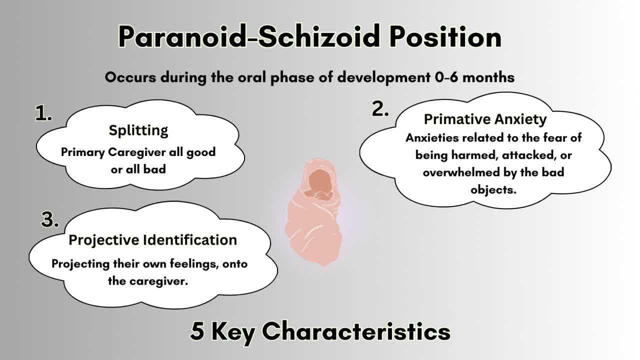 seem hostile or rejecting. another characteristic is emotional turmoil. the infant's emotions during this stage can be intense and volatile. they may experience both pleasure and discomfort, and the feelings can change rapidly. finally, at this early stage of development, the infant sense or self is not yet fully formed. they experience themselves and the world as fragmented. 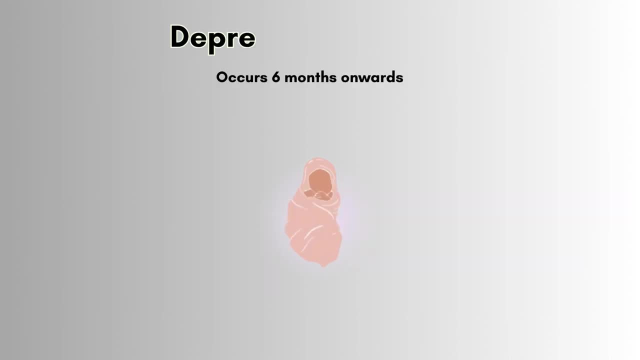 and undifferentiated. there are four key characteristics that occur during the depressive position, which occurs from six months onwards in the infant's life. as the infant's emotional development progresses, they move into the phase of integration. during this stage, the infant begins to integrate the good and bad aspects of their 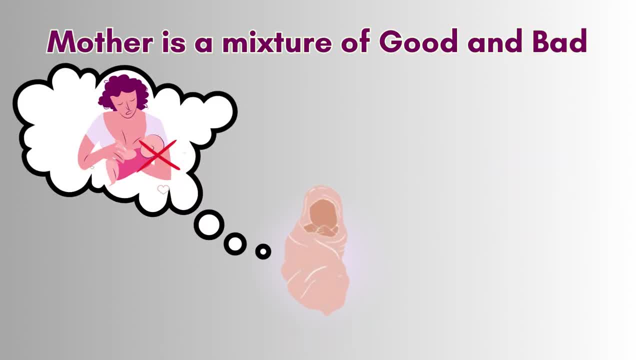 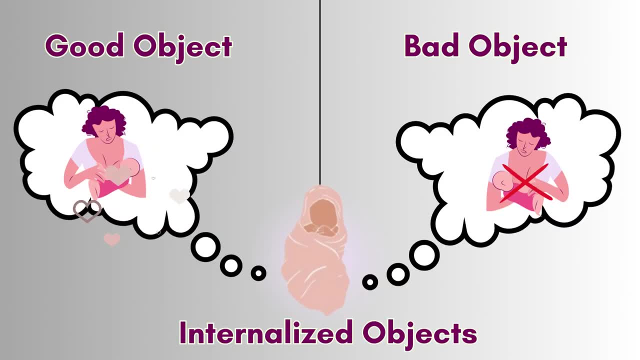 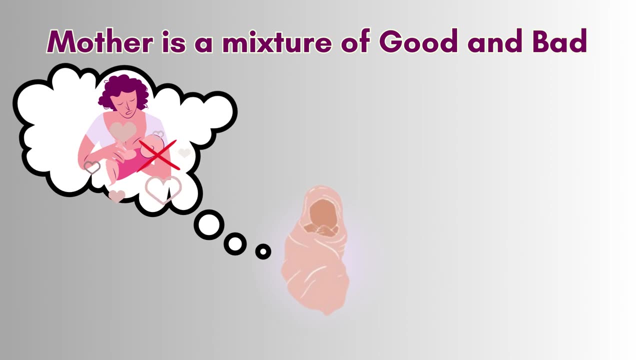 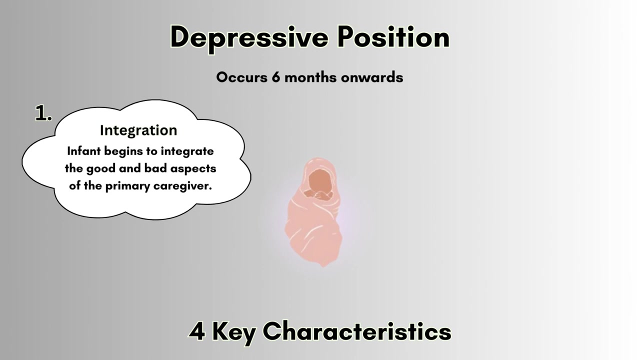 experiences with their caregiver, leading to a more complex and real, realistic understanding of relationships. so, instead of seeing the mother as all good or all bad, the infant is able to see that the mother is a mixture of both good and bad components. another key aspect of the depressive position is that the infant starts to develop a sense. 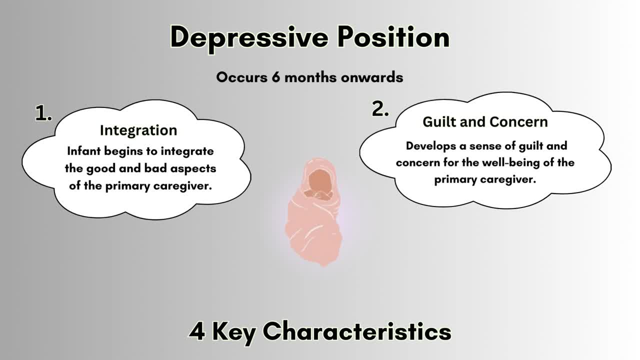 of guilt and concern for the well-being of their primary caregiver. the infant may feel remorse for their aggressive impulses, for example having angry feelings, for example, a持 없는罪. These are feelings towards their caregiver, and they may also start to fear losing their love and care as a consequence of them having showed angry and aggressive. 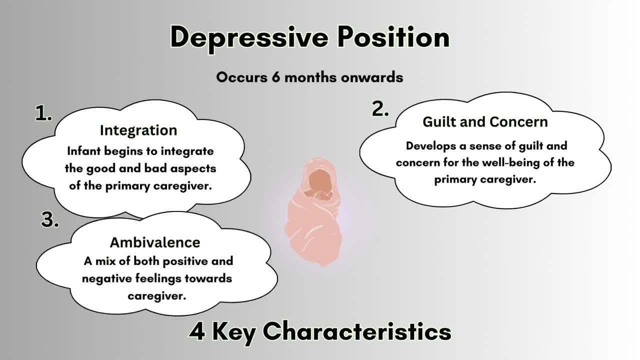 impulses towards their primary caregiver, the infants may also experience ambivalence. the depressive position involves a mix of both positive and negative feelings towards a caregiver. the infant experiences are more nuanced and layered view of their caregivers and the feel more strongly dependent towards the care giver. so, from your child to the best new Zoom synagogue based care giver, anyพyyс. 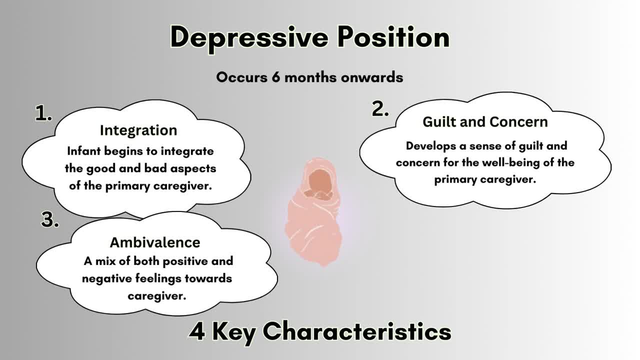 as they integrate both loving and angry feelings. And finally the infant will develop the capacity for whole-object relations. Through the depressive position, the infant begins to form whole-object relations where they can see caregivers as a complete and complex entity with both positive and negative qualities. 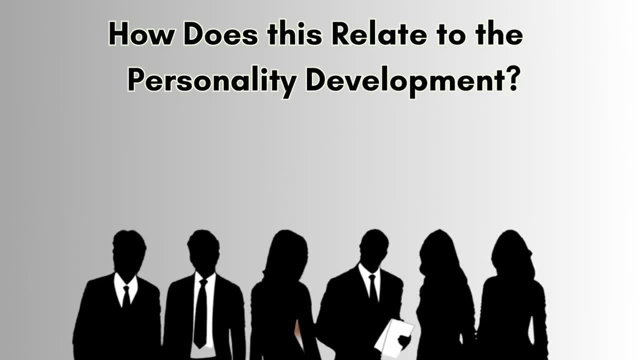 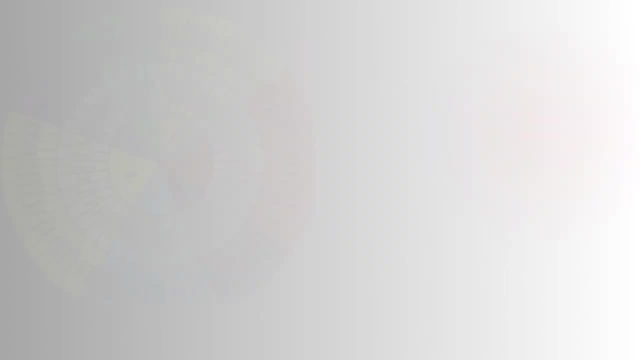 What we see from object relations theory is that the early stages of emotional development have a profound impact on how an individual's personality develops. These early views and responses to environmental emergencies shape how a person handles emotions and copes with stress as they grow older. 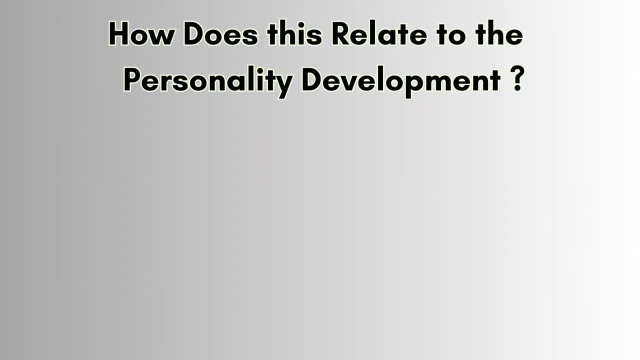 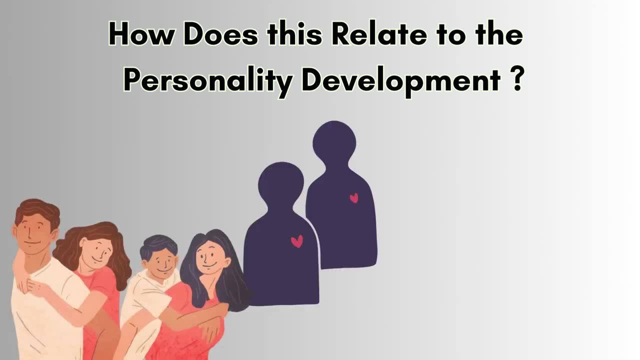 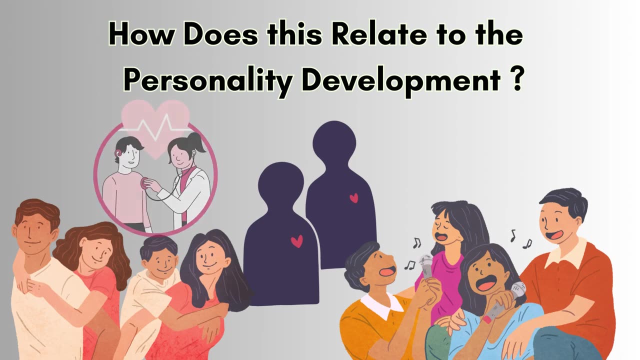 Detachment styles formed during these stages also influence a person's attitude to forming and maintaining relationships, which consequently leads to emotional development. Detachment plays a crucial role in shaping personality over time. Whilst secure attachments lead to healthier personality development, anxious or avoidant attachment styles can lead to difficulties.